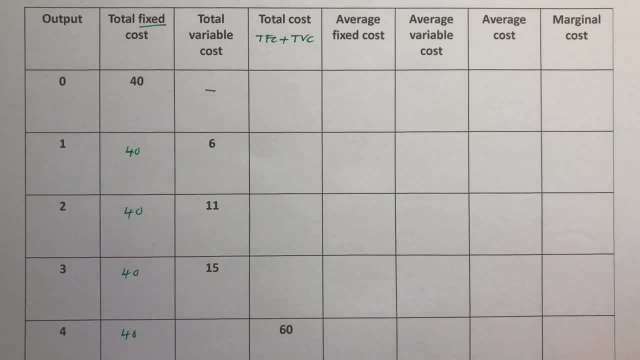 plus total variable cost. That's how you work out your total cost. So therefore, if this is 60, and we know that our total fixed cost was 40,, to find out what the variable cost is, it must be the total costs minus the total fixed cost will give us our total variable cost. 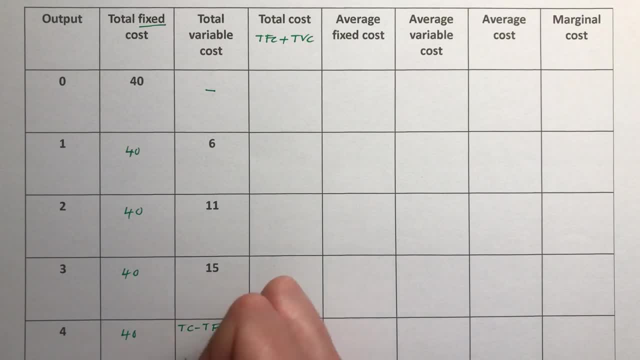 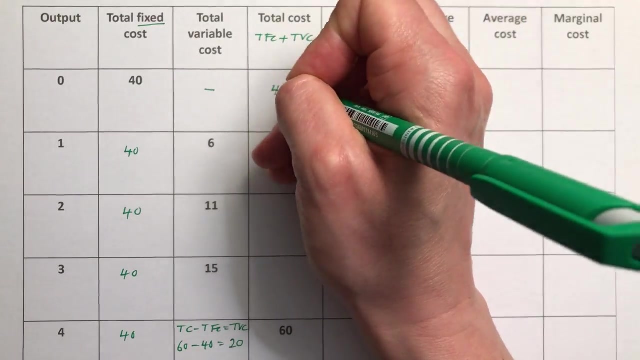 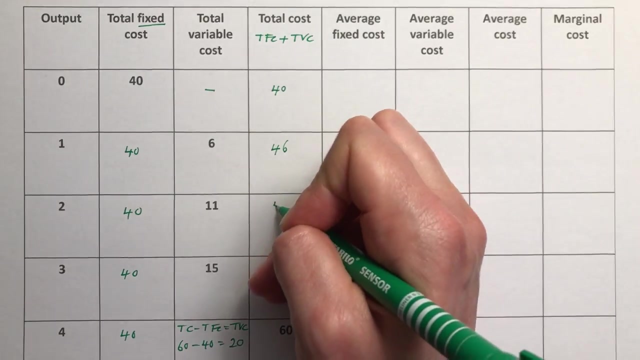 So in this case, total cost is 60, take away the 40, equals 20.. So then, to work out our total costs: when we don't have any output, it's 40 plus nothing. When we have one unit, it's 40 plus 6.. Two units: 40 plus 11.. Three units: 40 plus 15.. 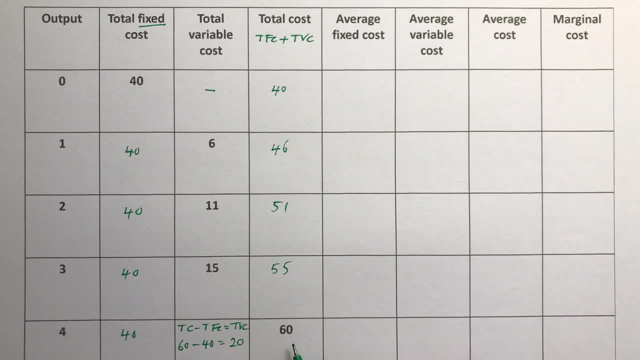 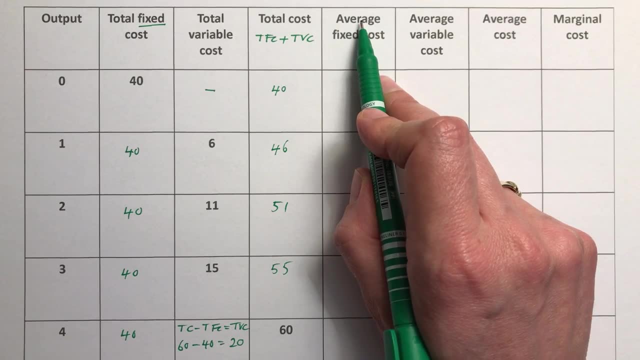 And then we know that when it's four units, it's 60.. The next one is the average fixed cost. If you have any average, you just need to divide it by the amount of output. If you have an average fixed cost, you just need to divide it by the amount of output. 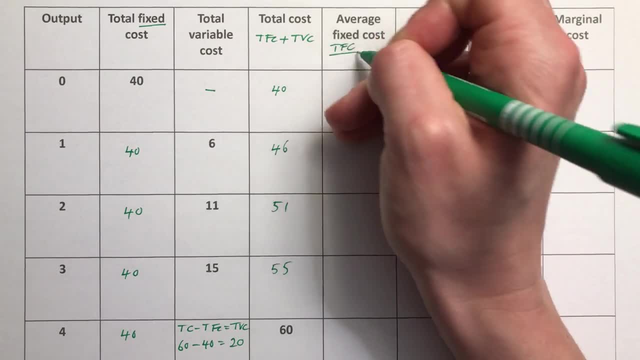 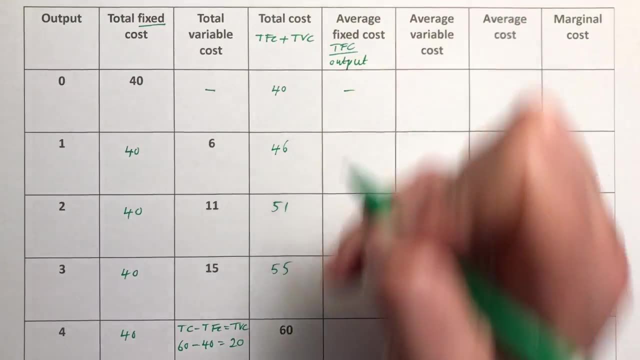 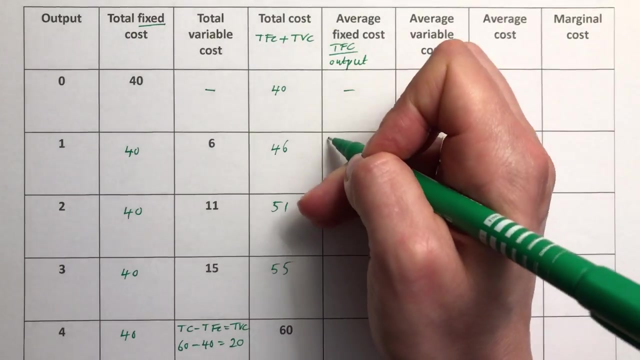 So this is going to be total fixed costs divided by output. The first one: we don't have any output, so we'll just put a dash for that, but the next one, our total fixed cost. here, total fixed cost is 40, and we have one unit of output. So 40 divided by 1 is 40. 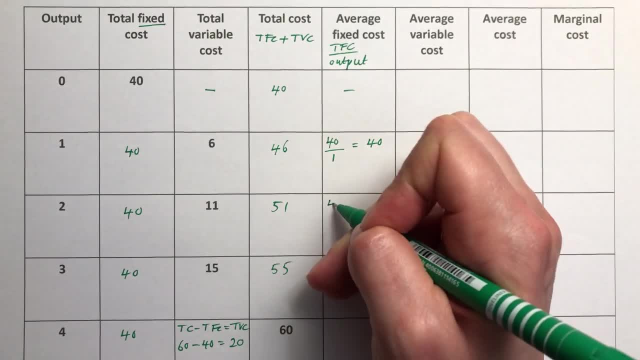 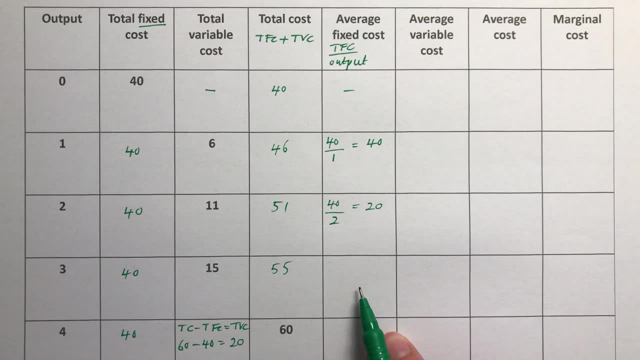 The next one: our total fixed cost is 40 again, because it always is and we have two units, so this is 20.. The next one: total fixed cost, again 40 divided by 3, and that one will be 13.3 recurring. 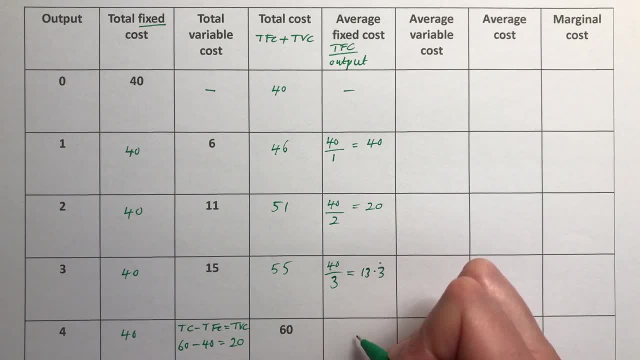 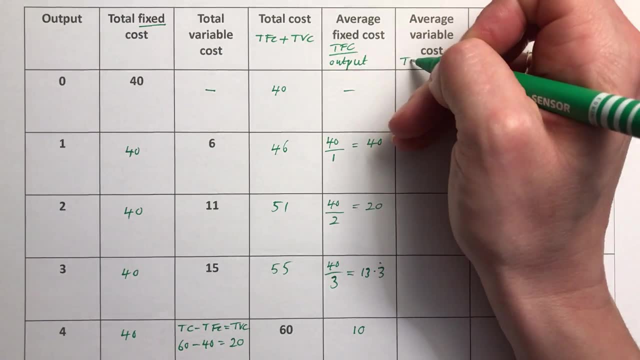 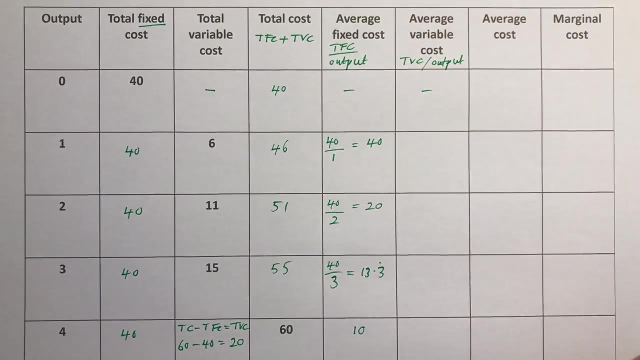 and four units. it will be 40 divided by 4, which is 10.. The next one: average variable costs. this is total variable cost divided by output. again the first one: no units, so we'll just put the dash in. then the next one, the total variable cost. these are: 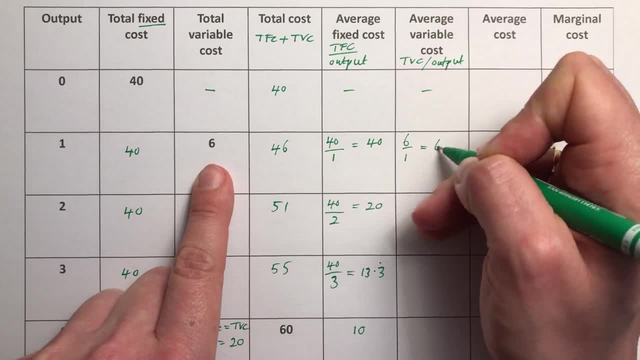 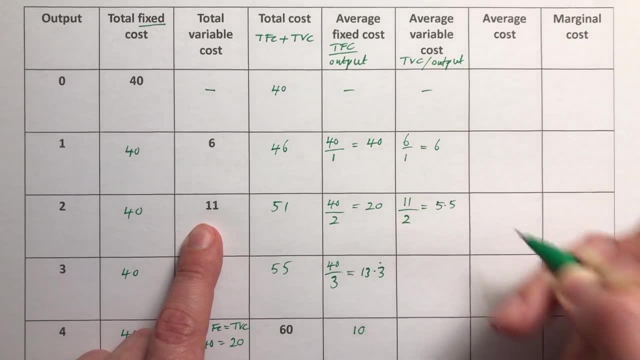 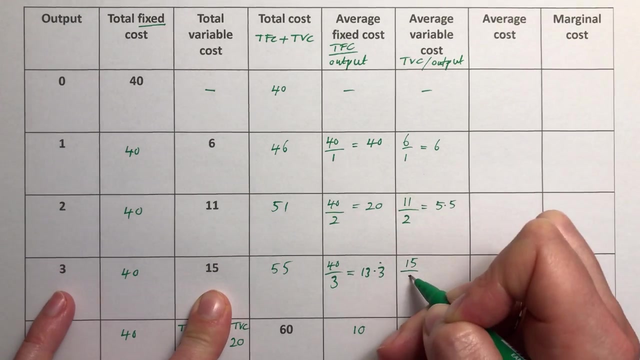 here. this is six divided by one, which is six, the next one, eleven, divided by two units, is five point five. the next one is 15. total variable cost divided by three units, which is five, and then for four units it's 40. sorry, it's not, it's. 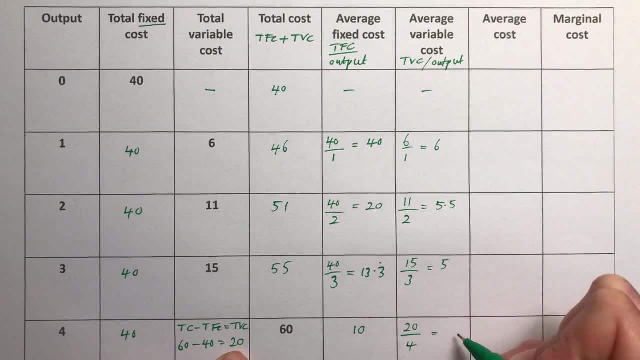 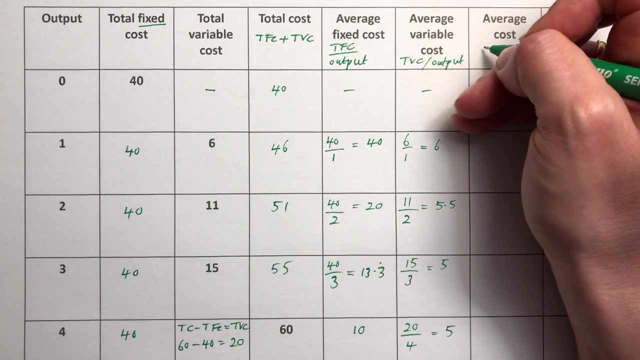 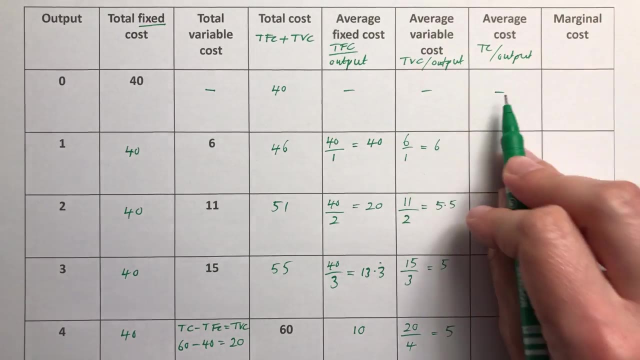 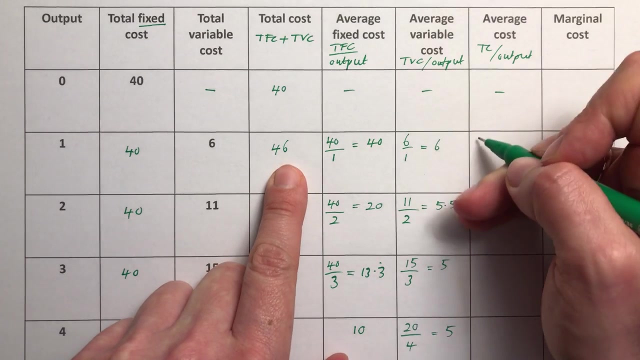 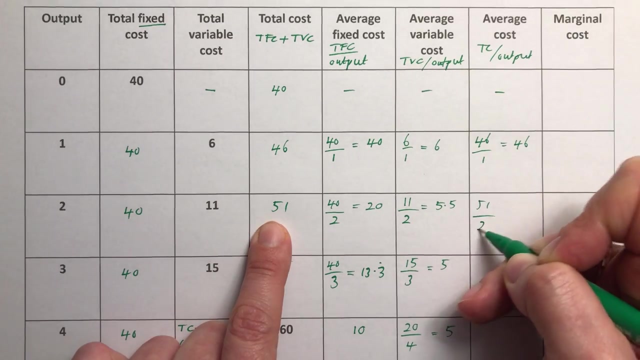 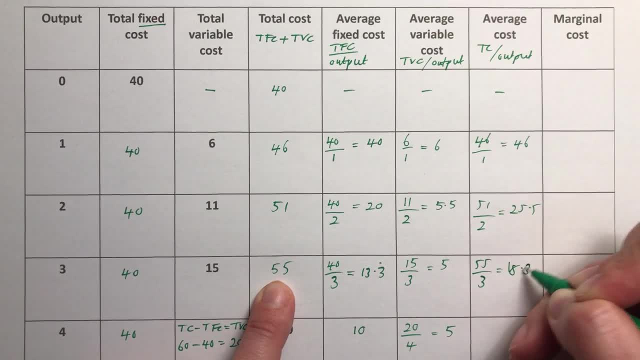 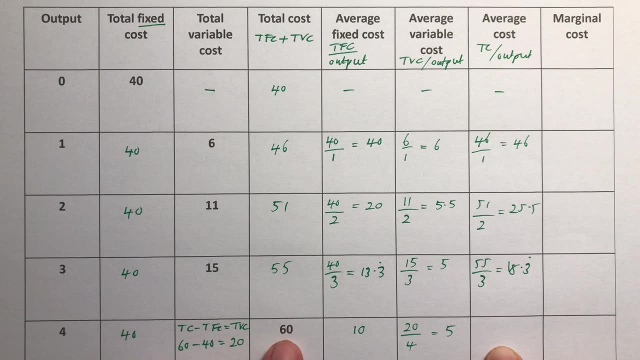 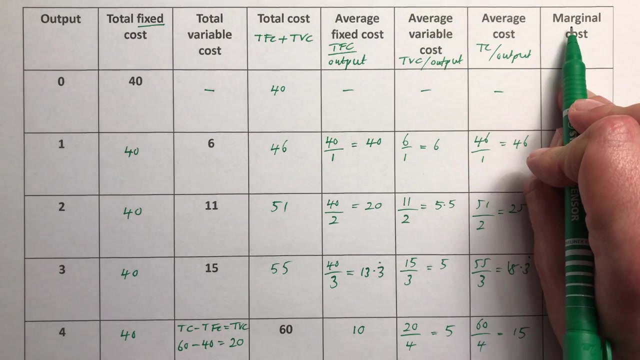 three units, which is 18.3, recurring, and then the last one, four units. your total costs here are 60, divided by 4 is 15.. then we get to marginal cost. this is the one that you might think. oh, what's that? remember, marginal means an additional amount. so this is saying: if you have an additional amount, 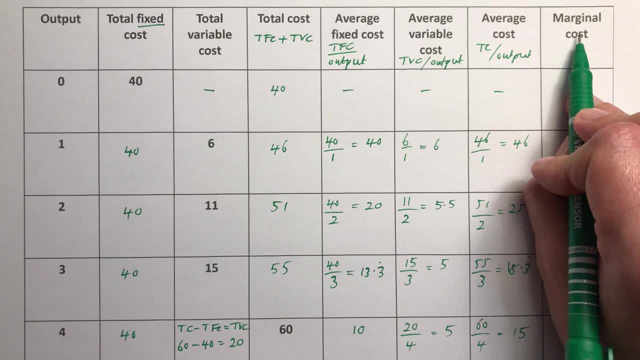 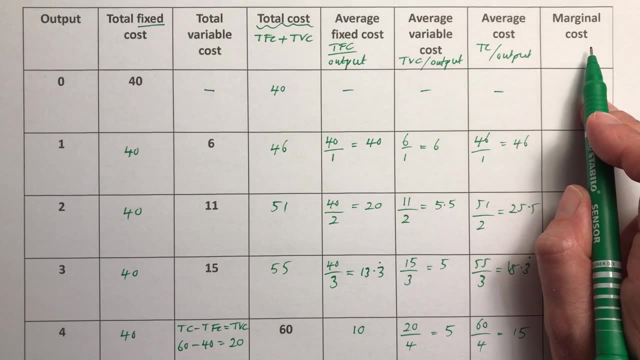 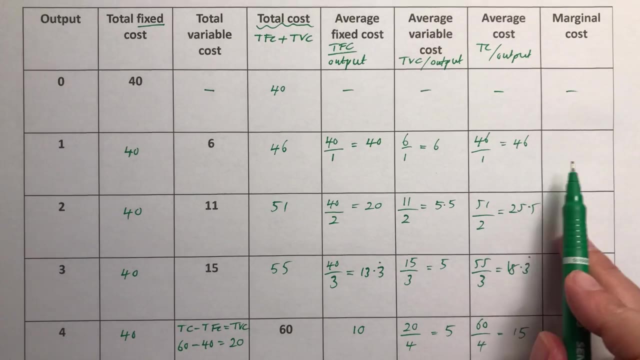 of output. how much do your total costs go up by? so your total costs are over here and you're looking to see how much they go up by when you make an additional amount or an additional unit of output. and again, here we're not producing any, but when we decide in the business to produce one. 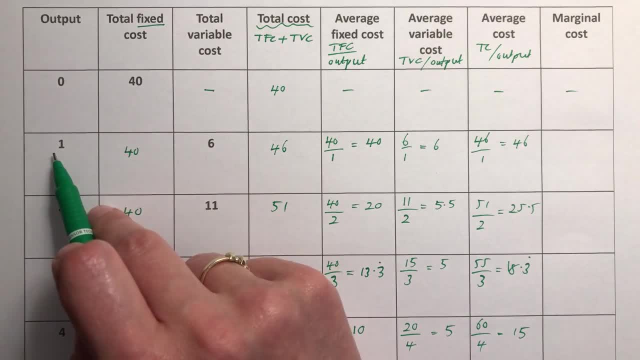 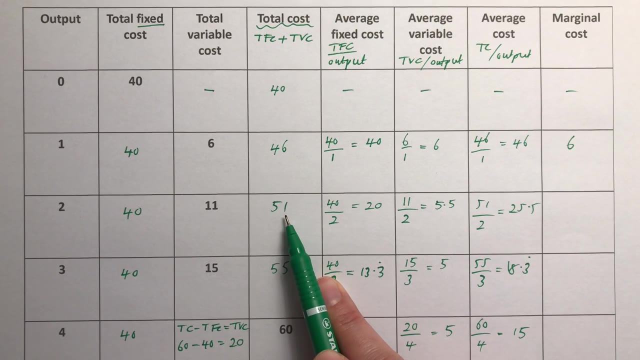 car rather than no cars, our total costs go from 40 to 46, so therefore our marginal cost was six. when we decide not to produce one but to produce two, our total costs go from 46 to 51 and therefore the marginal cost, the additional cost to the business of producing.